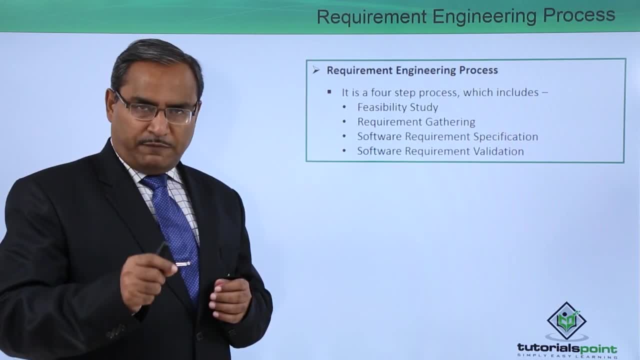 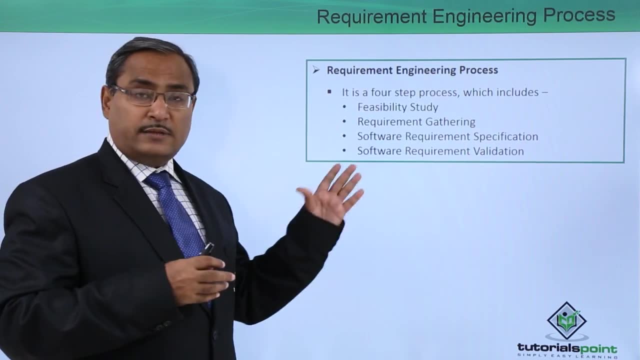 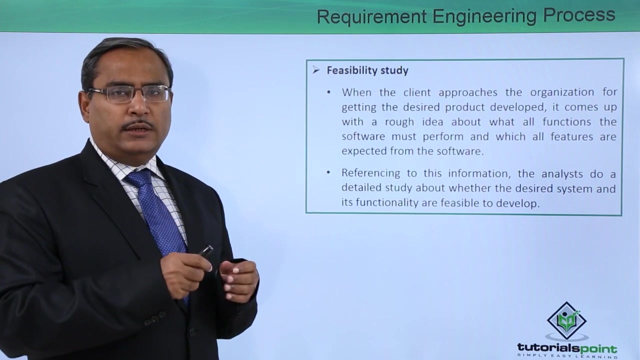 we shall go for software recoverment specification and then we shall go for software recoverment validation. So in this way we shall have our separate slides on each and every topic We are going with, starting with our feasibility study When the client approaches the organization. 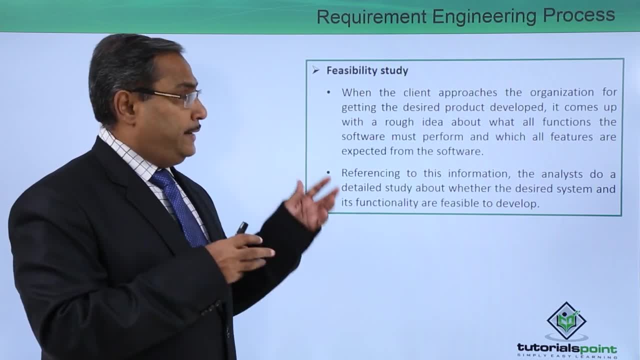 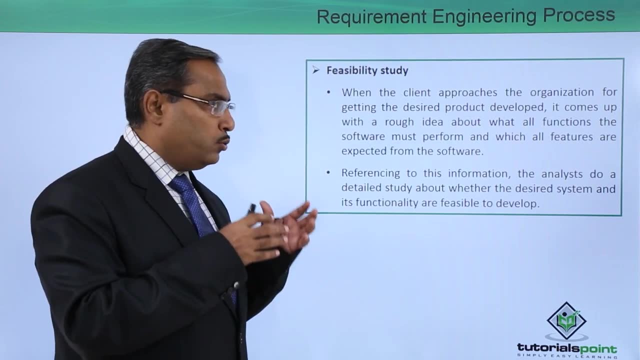 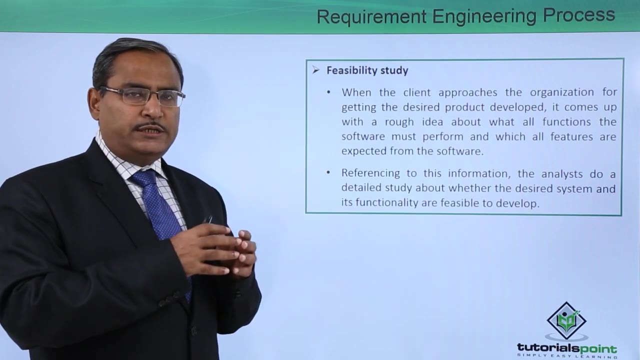 for getting the desired product developed. it comes up with a rough idea about what all functions the software must perform and what or which all features are expected from the software to get implemented. So in the initial discussion with the client, in the initial discussion with the customer, 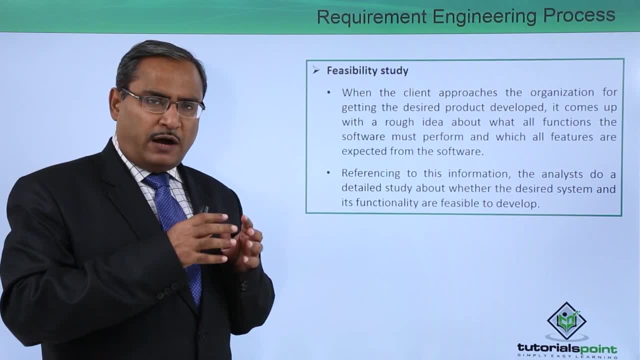 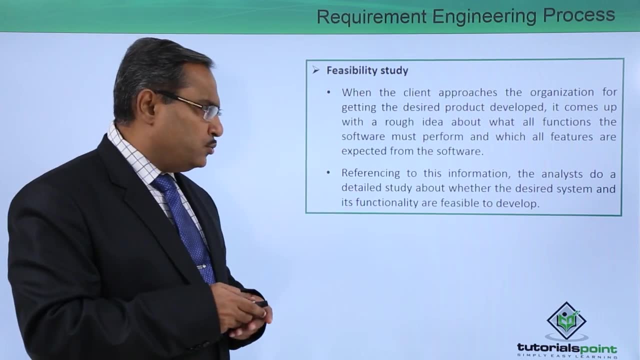 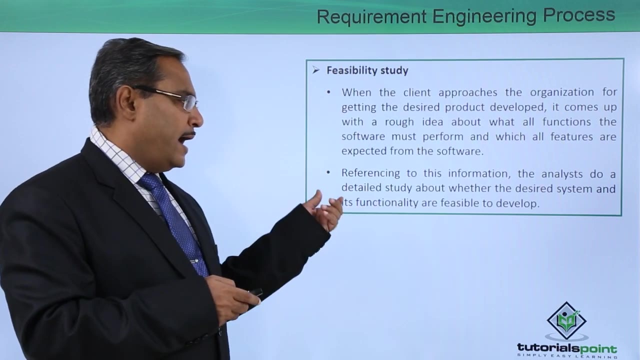 we shall be getting that, the rough idea regarding the what are the functions the software should do and what are the features the software should implement. So, referencing to this information, the analysis, do a detailed study about whether the desired system and its functionality are feasible to develop, And that will be done in our feasibility study. So we shall 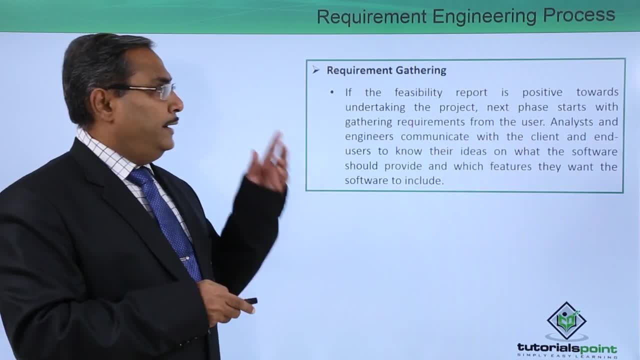 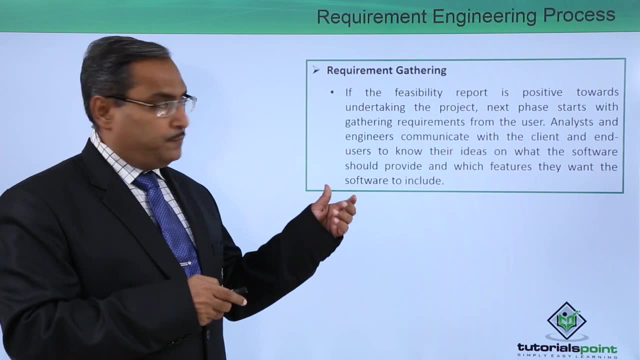 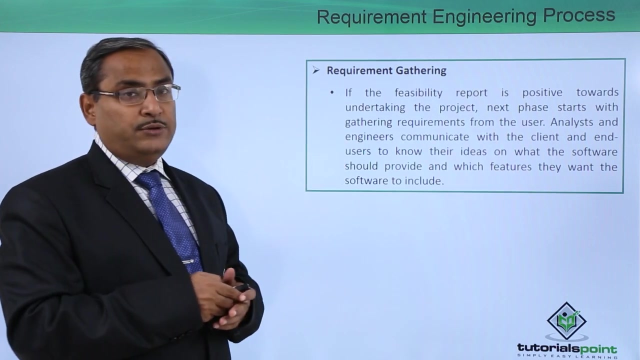 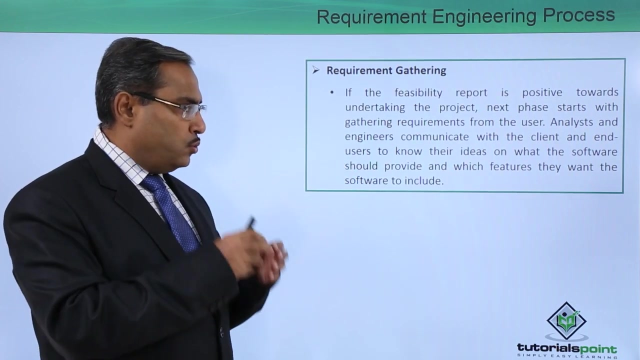 go for the next one, that is, our recoverment gathering. So if the feasibility report is positive towards undertaking the project, then the next phase starts with the gathering requirements from the user. So analysts and engineers communicate with the client and end users to know their ideas on what the software should. 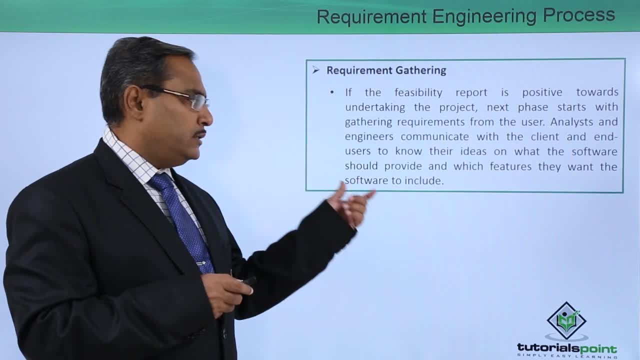 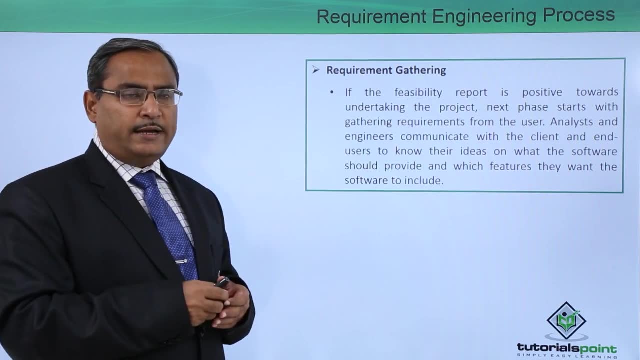 provide and which feature needs to be implemented. So if the feasibility report is positive, which features they want the software to include? so now they are going for the further detailing, doing further communication with the users, with the client, so that they can get the idea. 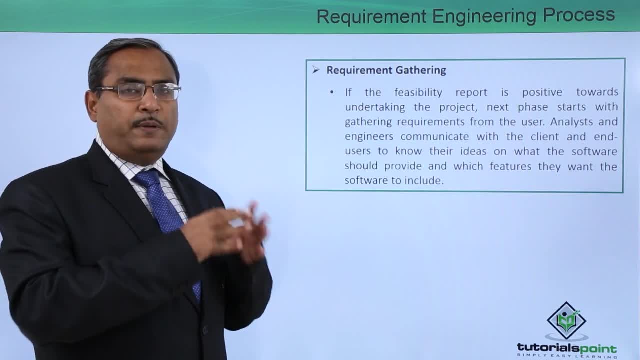 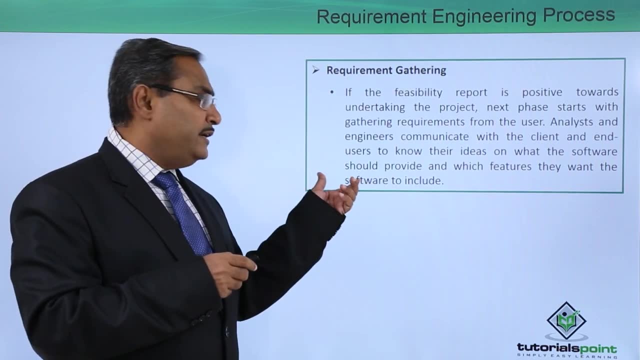 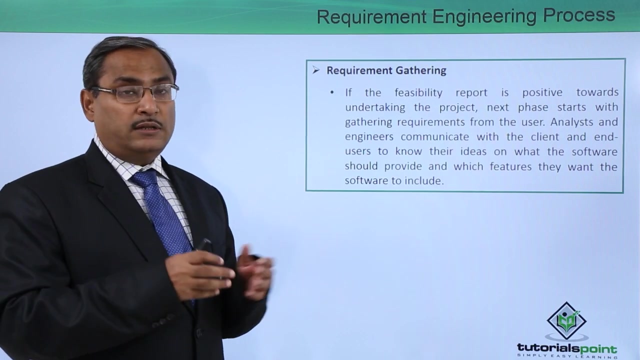 that after doing the feasibility study we got the report. let it be positive that will be taking this particular project. so now this recommend gathering will be done more, more into the details so that the software can be developed. we know that. what are the functionalities to be implemented and what are the features will be there in the software. next one is: 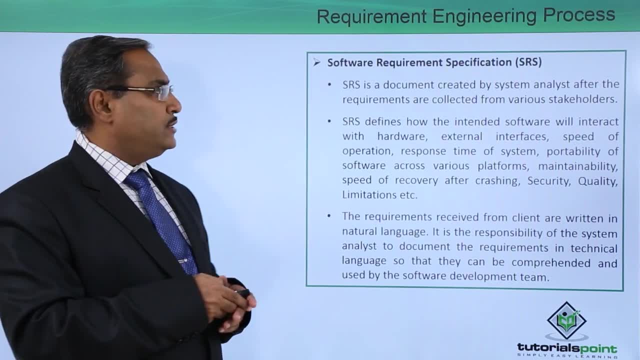 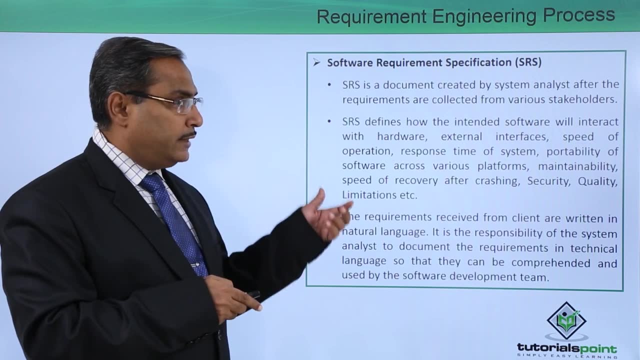 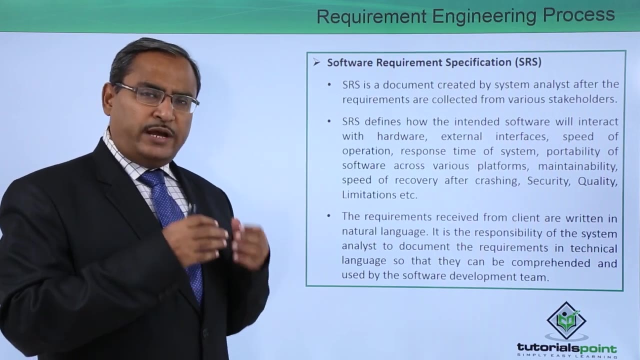 our srs, that is, the software requirement specification. so srs is a document created by system analysts after the requirements are collected from various stakeholders. we discuss this. stakeholder was the meaning of this stakeholder. so stakeholder means those persons who are positively or negatively affected by the execution of the project. 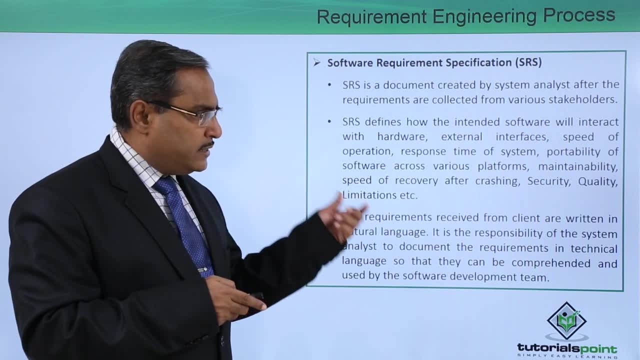 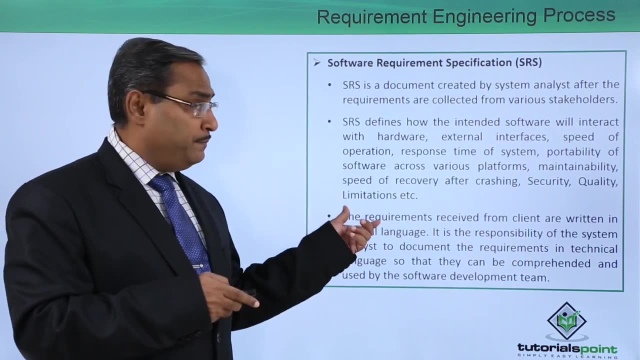 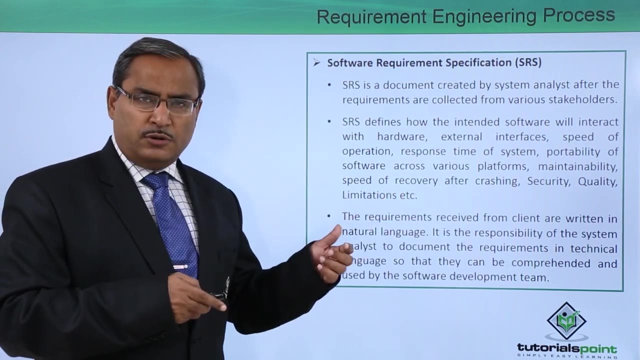 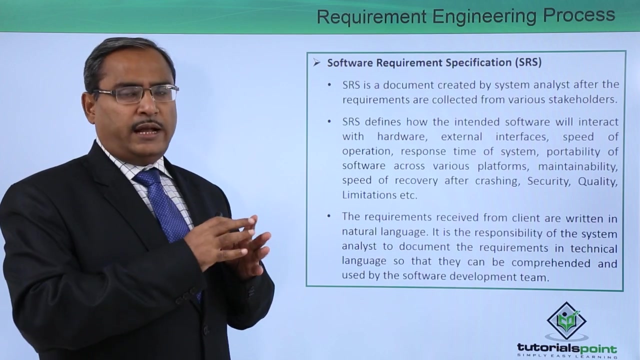 so srs defines how the intended software will interact with the hardware: external interfaces, speed of operation, response time of the system, portability of the software across different platforms. what is the platform? platform means the software, that is, the operating system, and the respective hardware. in combination of them, we can, we can call it as the platform. 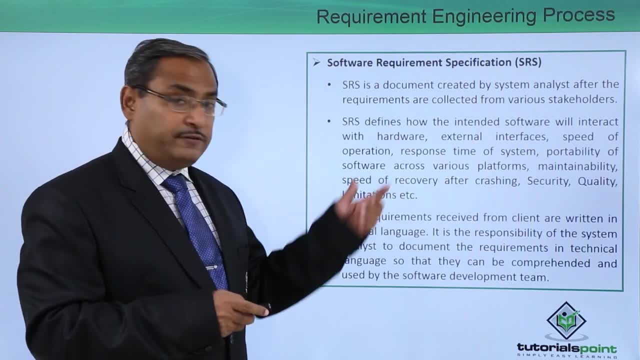 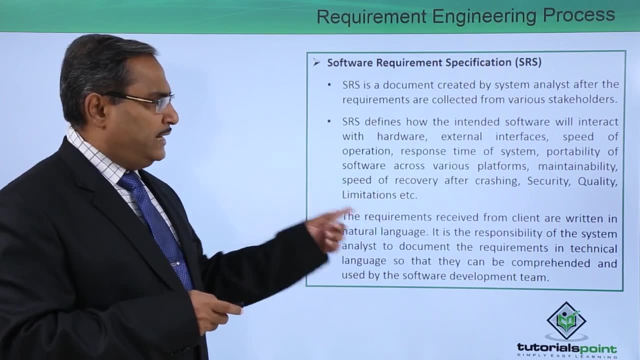 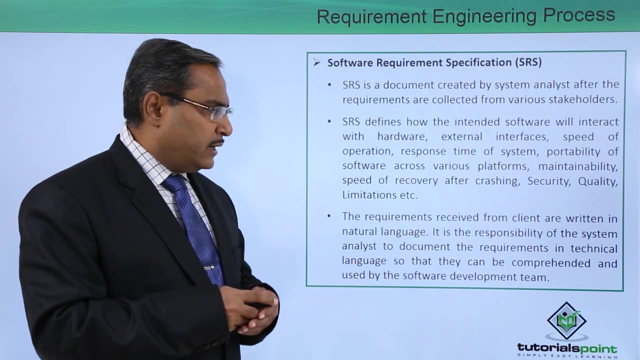 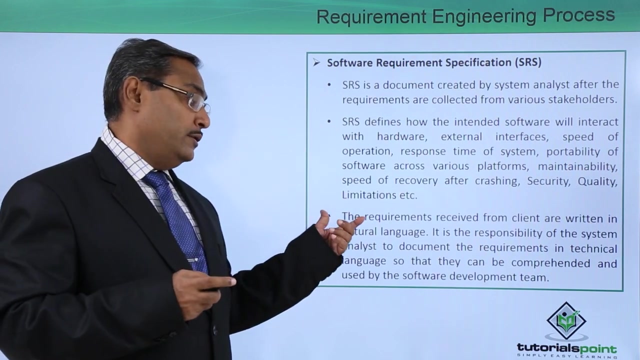 and then maintainability, speed of recovery after crashing, security, quality limitations, etc. so all these things will be kept in a proper documentation and that is our srs. so the recommends received from the client are written in natural language. so whatever the language you are considering, so that will be written that one. it might be english or some other languages also, but 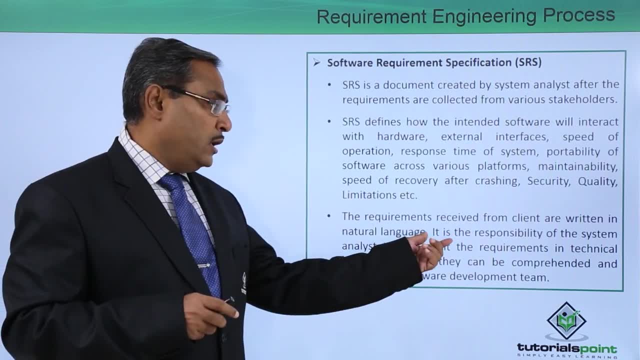 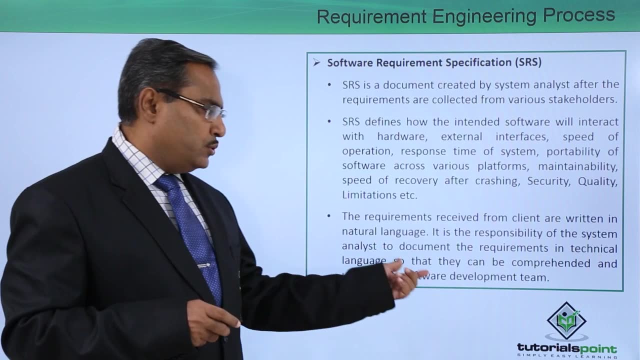 it is not a programming language. so that i can assure you, this is the srs under i ss and that is the srs under i don't speak Kannada. so it is the responsibility of the system analyst to document the recommends in technical language so that 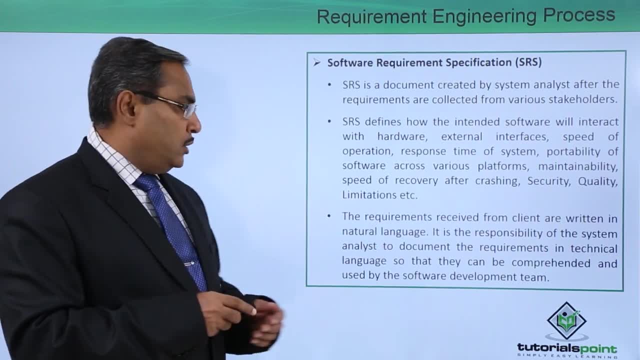 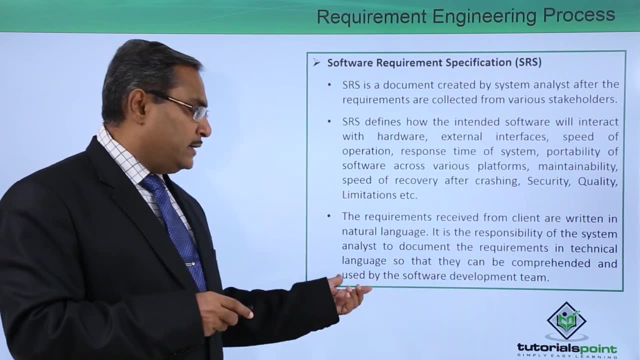 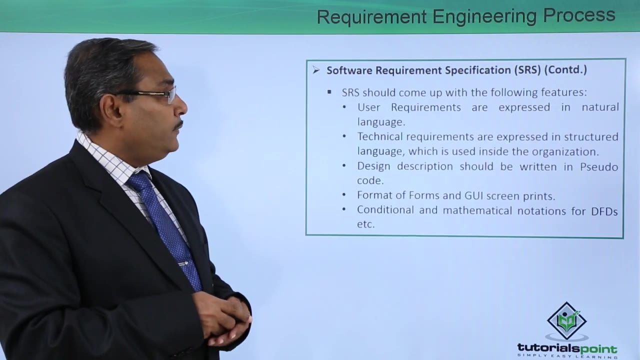 they can be comprehended and they have been comprehended and used by the software development team. so in this particular case we can also use some technical language so that it can be comprehended and can be used by the software development team. so that is the language of. 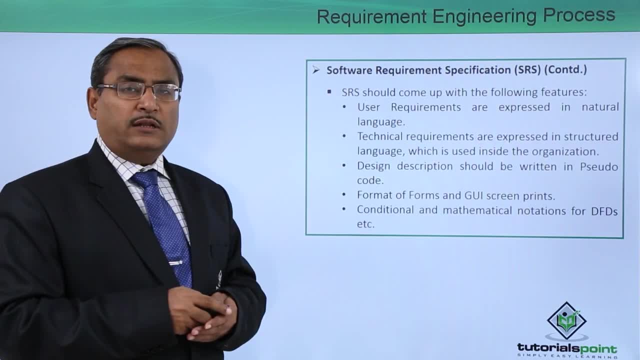 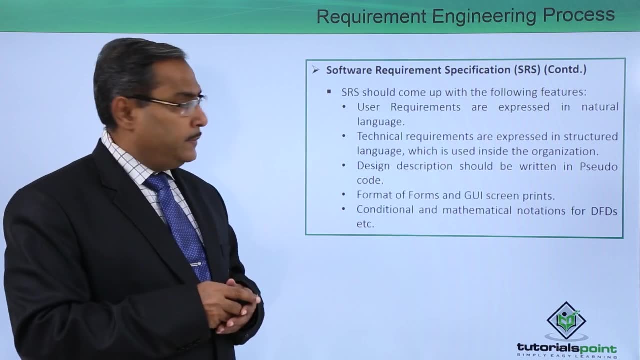 this srs. These are the- should come up with the following feature. so what are the features it should have? So user requirements are expressed in natural language. technical requirements are expressed in structured language which is used inside the organization and then design description. 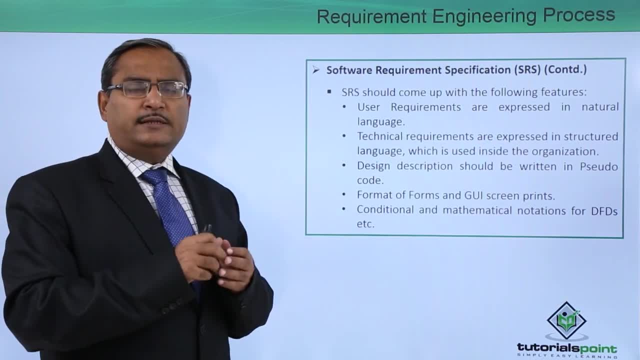 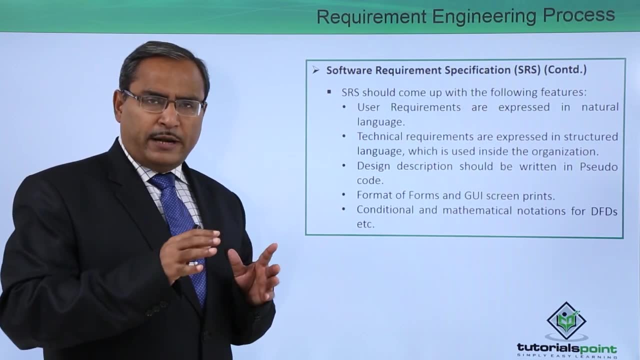 should be written in some pseudo code, that is, in some algorithmic form. it will be written in some pseudo code. we know that in case of pseudo code it is language independent. we are not maintaining any kind of syntax. what is the meaning of the term syntax means? 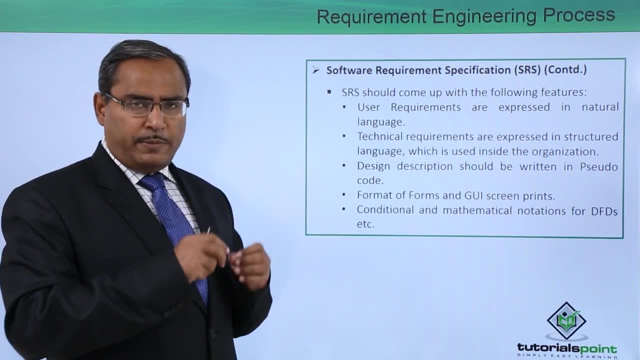 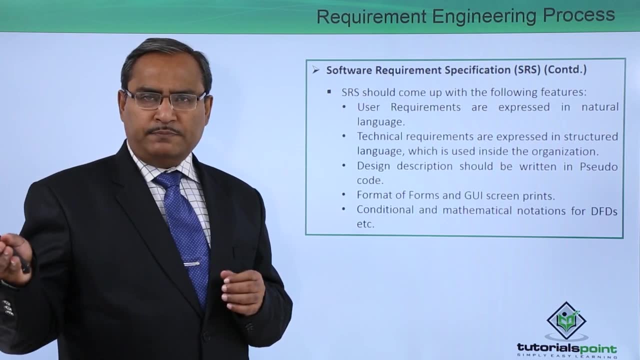 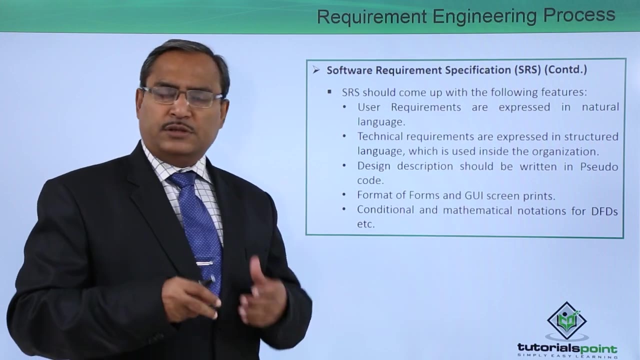 the grammar that means here we will be writing this particular recommend in some technical pseudo code So that the developer can implement that one when the phase will come. so it will be written in some syntax free pseudo code. and then format of the forms and the GUI screens. 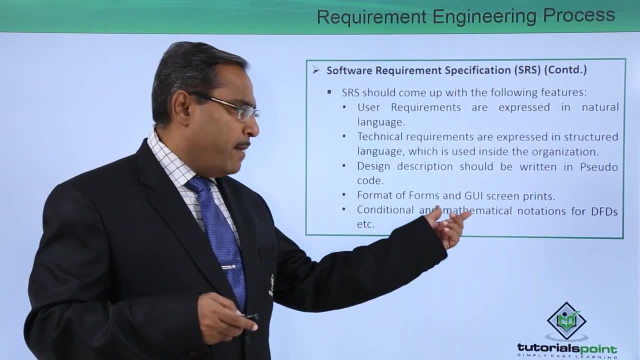 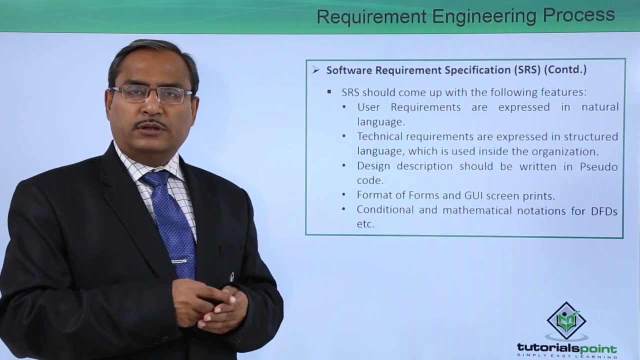 the prints will be made and then conditional and mathematical notations for DFDs and etcetera. So DFD means data flow diagram. so we are having a separate video on the DFDs. you can easily go for that- and we are also having a separate video on the pseudo code and all. 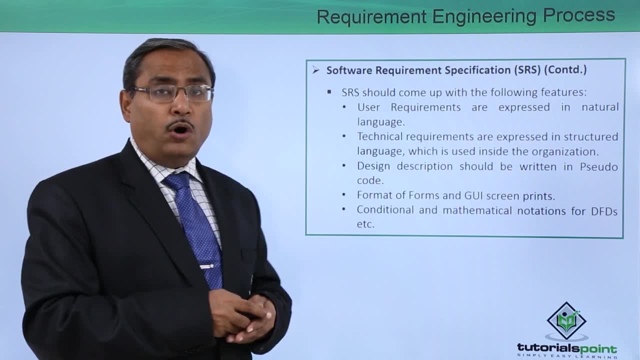 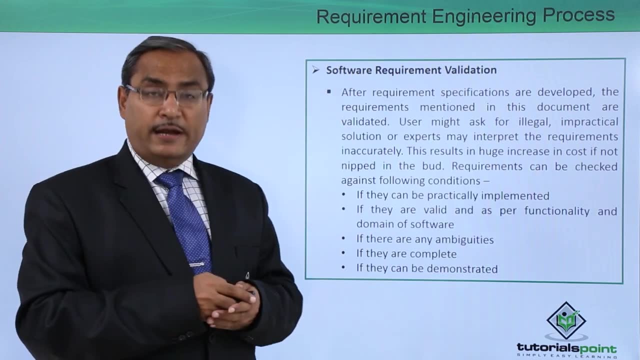 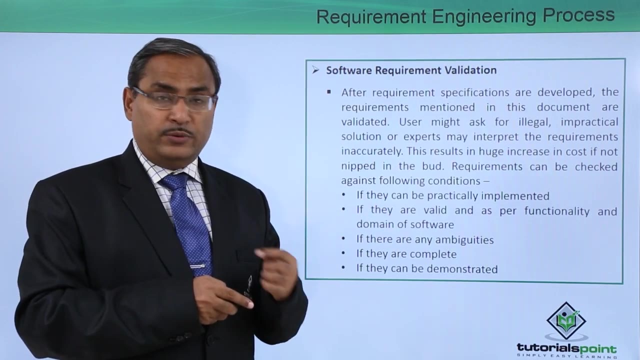 so these are the different. the SRS should contain all these things. Now we are going for the last phase, that is, the software recommend validation. so that is the fourth one. what were the earlier three? one? so first one was feasibility study. we discussed that one. 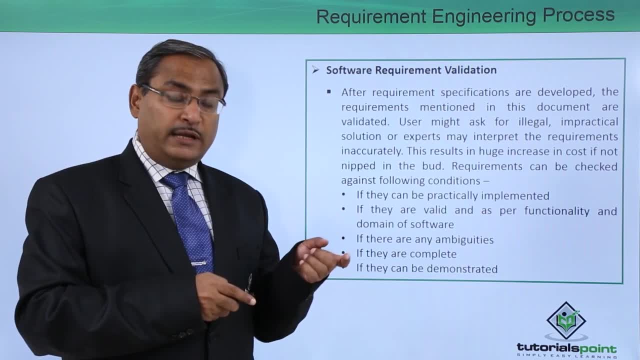 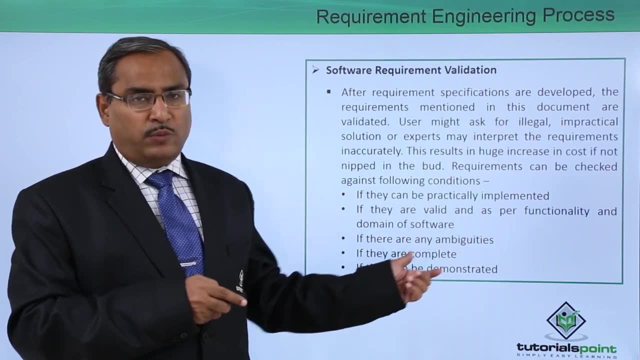 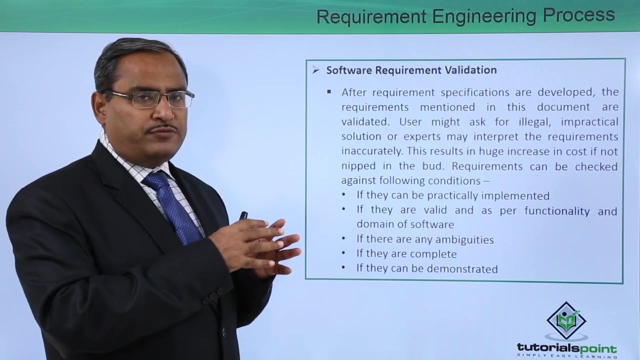 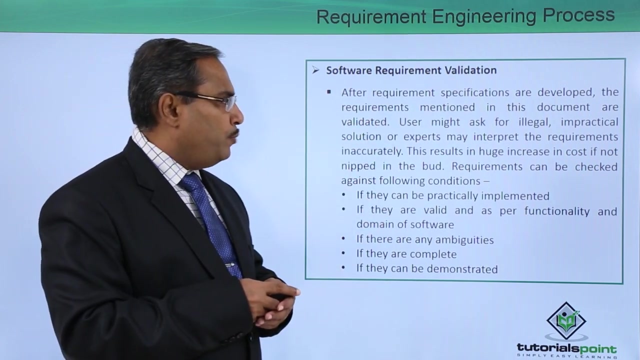 The next one was recommend gathering, and the third one was software recommend specification- SRS- and the fourth one is software recommend validation. so, all after arranging all these things in the software recommend specification, software recommend specifications are developed. the requirements mentioned in the document are validated. 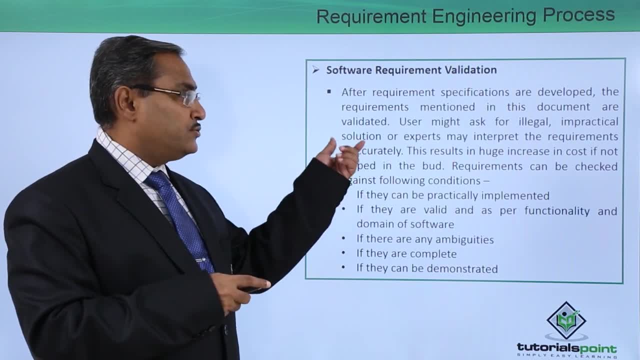 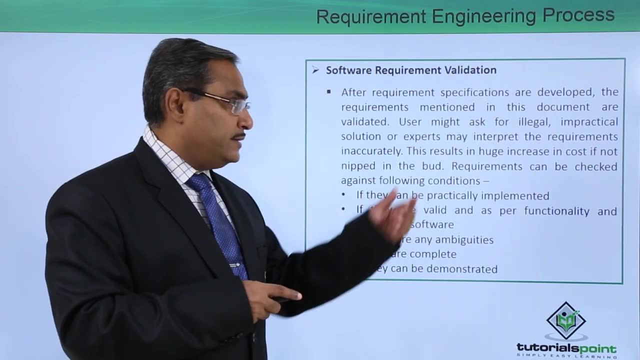 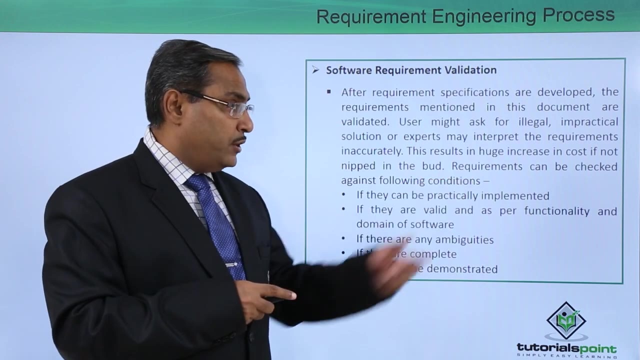 So user might ask for legal impractical In practical solutions or experts may interpret the requirements inaccurately. so this result: this results in huge increase in cost if not nipped in the bud. So that is why recommends can be checked against following conditions: 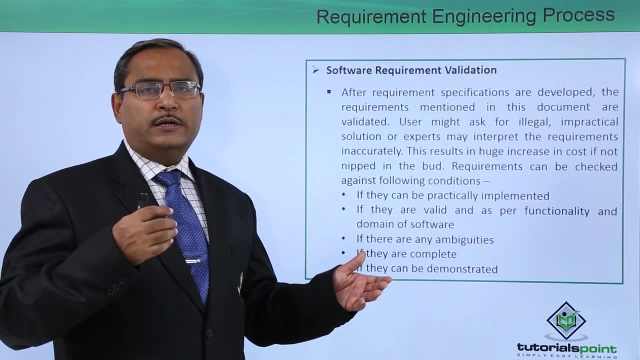 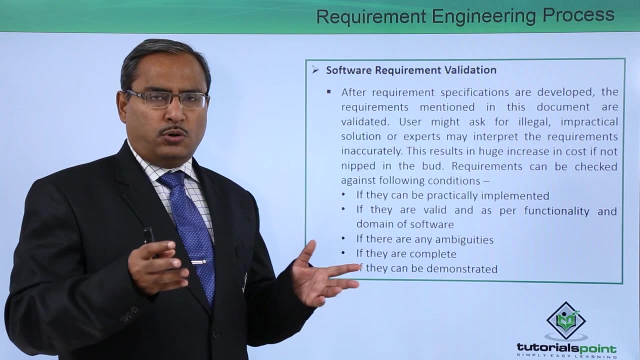 So what about the requirements we had? we have maintained that one in the properly documented way, in the form of DFDs, in the form of some natural language, in the form of some pseudo codes in our SRS. but here I should have to check whether really they are validated.